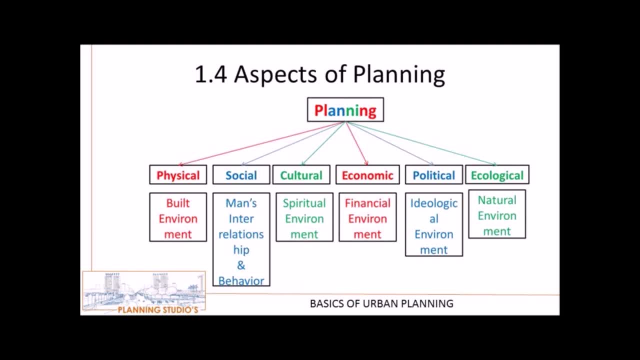 First is physical, aspect, which deals with the built environment. Second is social, deals with the interrelationship and behavior with surrounding. Third is cultural, deals with the spiritual environment of any areas. Fourth is economic, dealing with the financial environment. Fifth is political, dealing with the ideological environment that ensures stability of area. 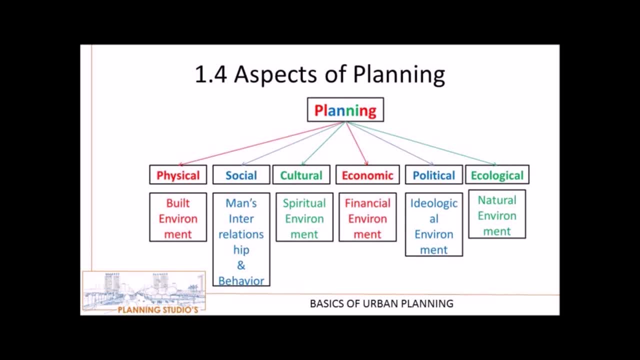 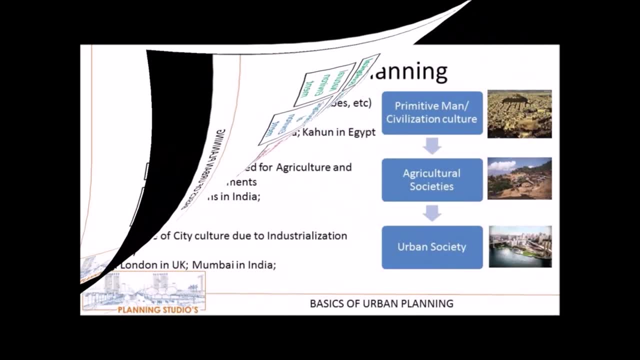 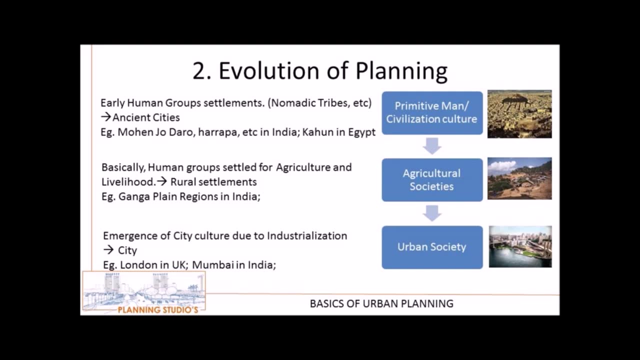 Last is ecological deals with tenational environment around the area. Hence planning is a multisectoral and multidimensional thing to exist. Planning is evolved since ancient times, But it progressed very slowly as earlier phase, and fast and later. The general evolution of planning is characterized by simple three-step. 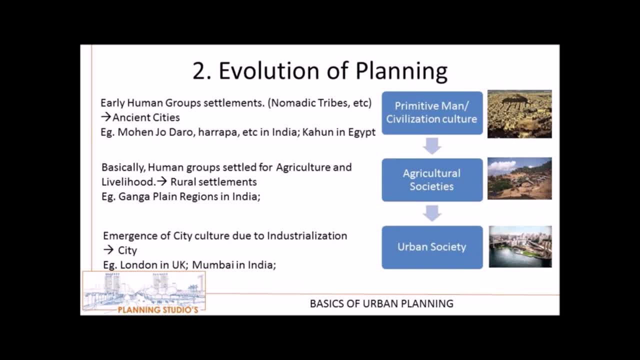 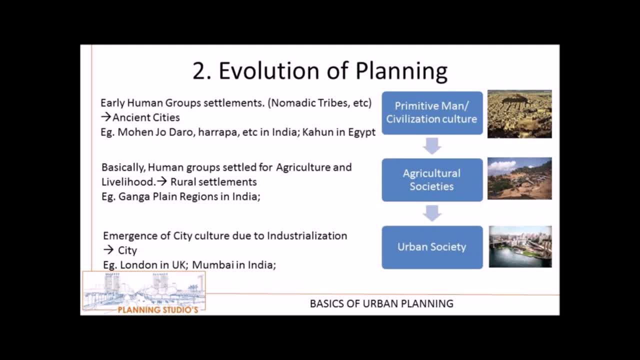 years ago. Early human group settled by 6000 to 3300 years ago, as humans ists imagined in terms of background. Early human group settled by 1000 to 3000 years ago as they have: Carmen, 2520 BY Early human group 6529 and to 1330, September, all besser. 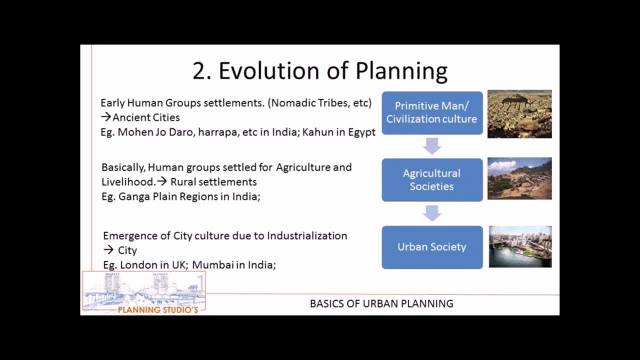 than common people. The United States, Ap canvi Moon and Lord Star, Applined Can thread in 303th century BC by Samison Frank and fellow으 entss Riot, British period 1901–3053.. Some of examples are Mohenjo- прис495 and Harappa in Indus valley, Gahan in Egypt, etc. 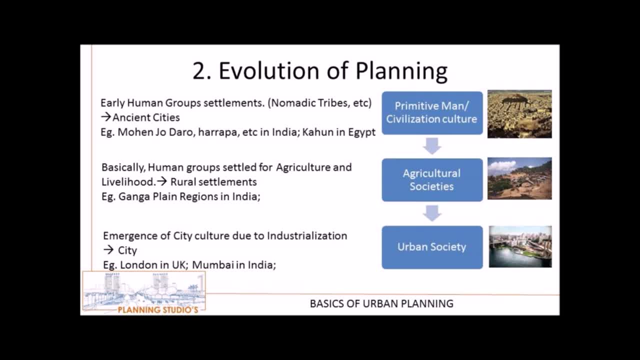 Then the settlers routed for agriculture activities and settled around the water resource areas. Example is Ganga plain regions of India. Lastly, the Western culture and industrialization. respecto al строiels in India句 phases to emigre. new town to serve the changed conditions. 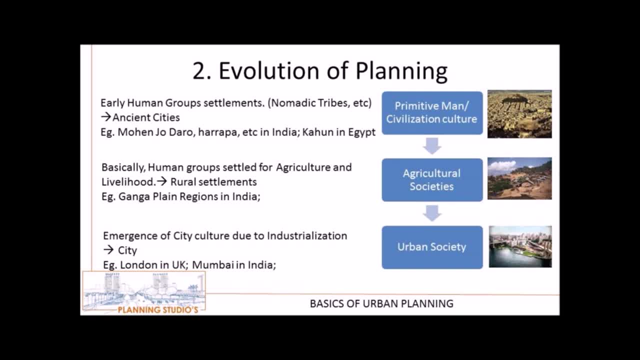 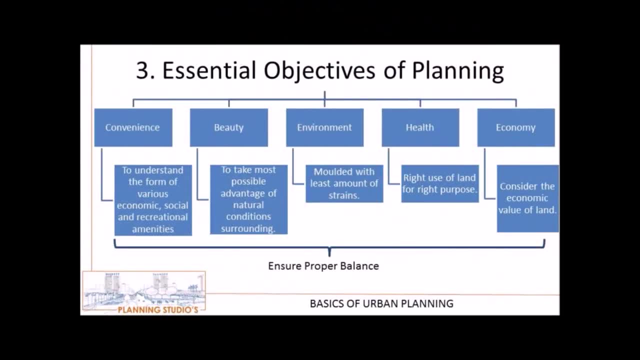 Such new town termed as urban societies in modern era. Thus, evolution of planning is very simple, precise in terms, by complex in its character. Some of essential objectives of planning are: 1. Convenience – to understand the form of various economic, social and recreational 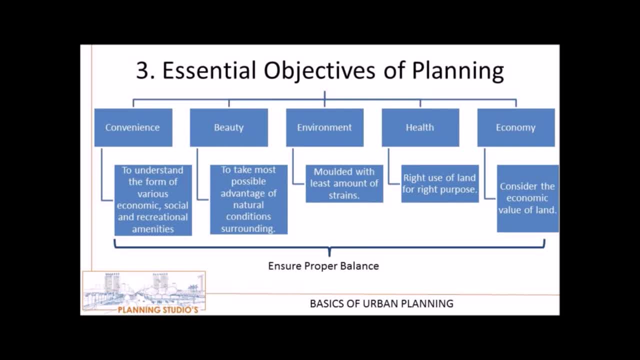 amenities. 2. Beauty – to take most possible advantage of natural conditions surrounding. 3. Environment – molded with least amount of strains. 4. Health – right use of land for right purpose. 5. Economy – consider the economic value of land.